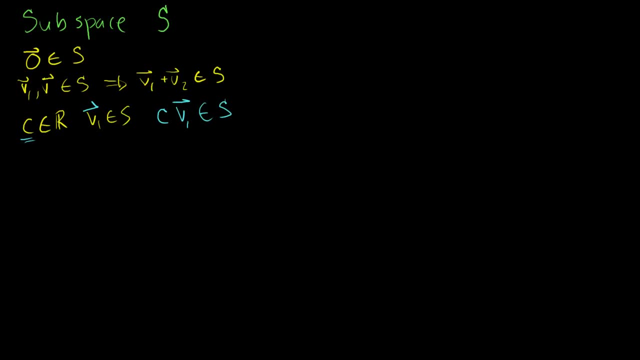 need to be true. Now let's see if we can do something interesting with what we understand about matrix Matrix vector multiplication. Let's say: I have the matrix A, I'll make it nice and bold, And it's an m by n matrix. 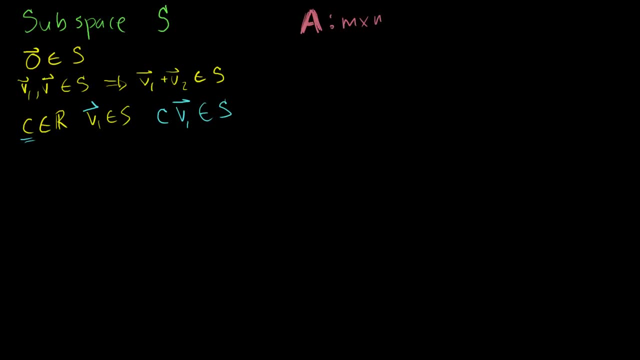 And I'm interested in the following situation: I want to set up the homogeneous equation And we'll talk about why it's homogeneous. Well, I'll tell you in a second. So let's say, we set up the equation. my matrix, A times. 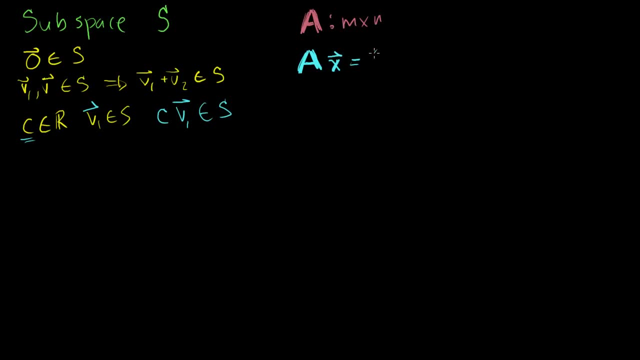 vector x is equal to the matrix, It's equal to the 0 vector. This is a homogeneous equation because we have a 0 there. Homogeneous. And I want to ask the question: I talked about subspaces. If I take all of the x's, if I take the world, the universe, 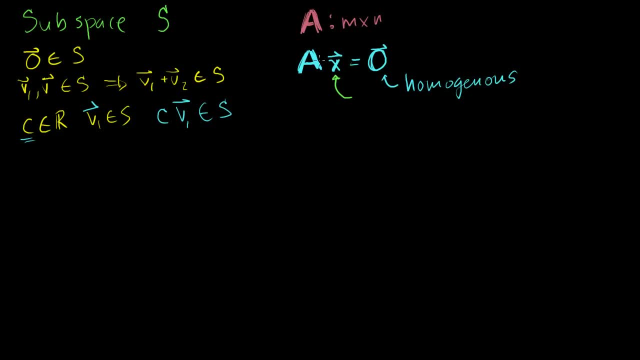 the set of all of the x's that satisfy this equation, do I have a valid subspace? So if I take- let's think about this- I want to take all of the x's, All of the x's that are a member of Rn. 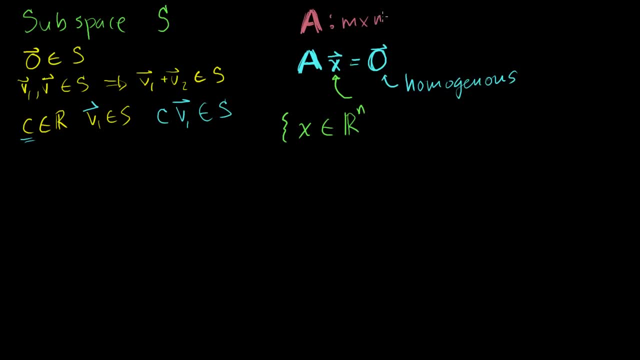 Remember, if our matrix A has n columns, then I've only defined this matrix vector multiplication If x is a member of Rn, if x has to have exactly n components, only then is it defined. So let me define a set of all of the vectors that are a: 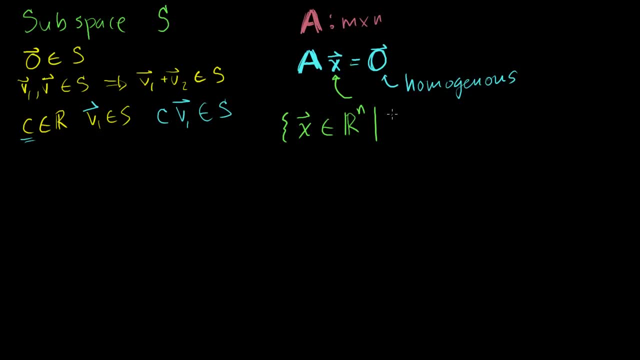 member of Rn. where they satisfy the equation A times my vector x is equal to 0.. So my question is: is this a subspace? Is this a valid subspace? So the first question is: does it contain the 0 vector? 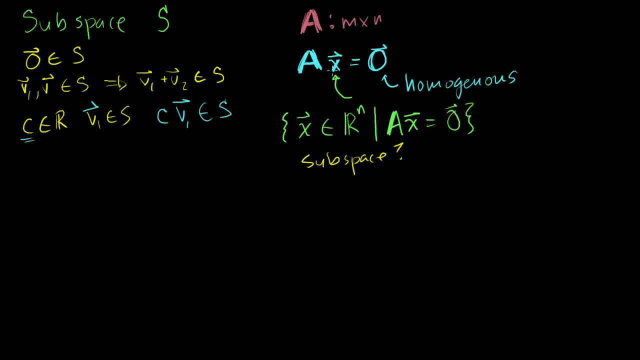 Well, in order for this to contain the 0 vector, the 0 vector must satisfy this equation. So what is any m by n? matrix A times the 0 vector. I'll write it like that: Times the 0 vector. Let's write out my matrix A. 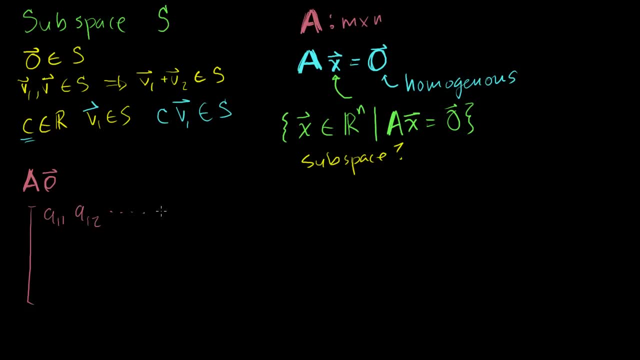 a11,, a12,, all the way to a1n. And then this: as you go down a column, we go all the way down to am1.. And then, as we go all the way to the bottom right, we go to. 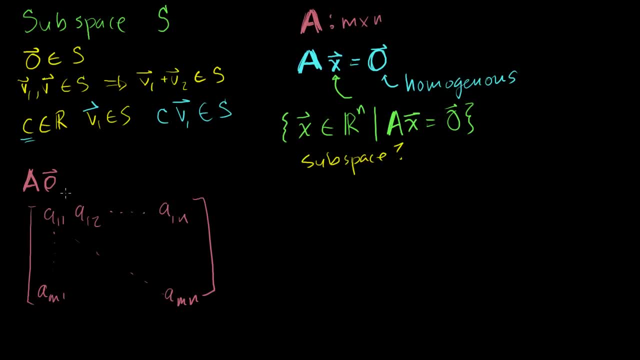 amn, And I'm going to multiply that times the 0 vector. that has exactly n components. So the 0 vector with n components is 0, 0, and you're going to have n of these. The number of components here has to be the exact same. 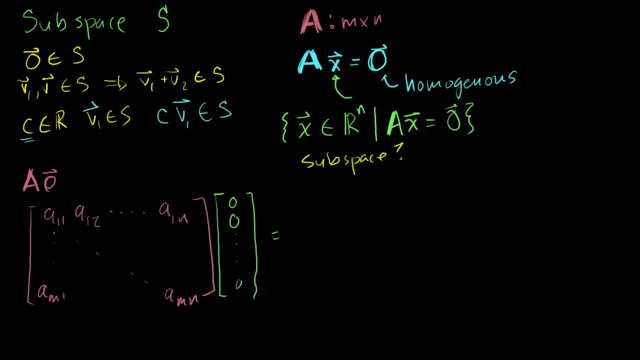 number of columns you have. But when you take this product, this matrix vector product, what do you get? Well, this first term up here is going to be a11 times 0 plus a12 times 0, plus each of these terms times 0.. 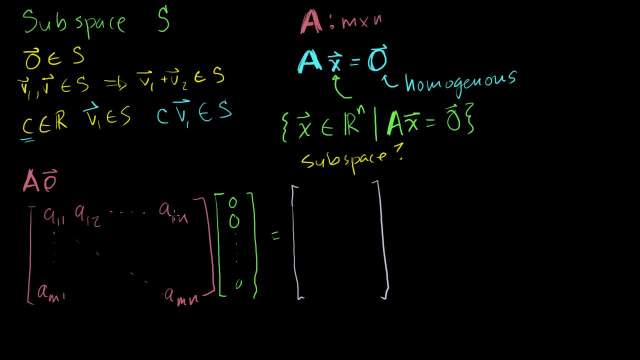 And you add them all up: a11 times 0 plus a12 times 0,, all the way to a1n times the 0. So you get 0.. Now this term is going to be a21 times 0.. 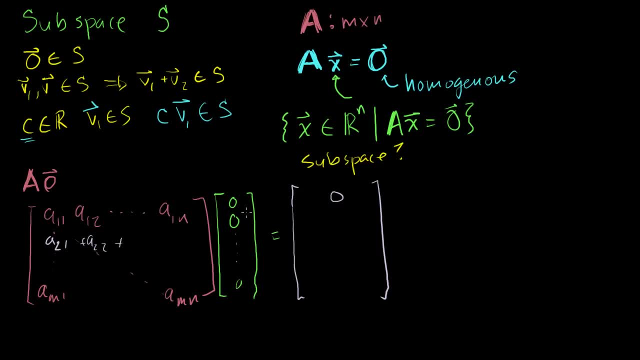 0 plus a22 times 0 plus a23 times 0, all the way to a2n times 0, well, that's obviously going to be 0. And you're going to keep doing that because all of these are essentially- you can kind of view it as the dot product of: 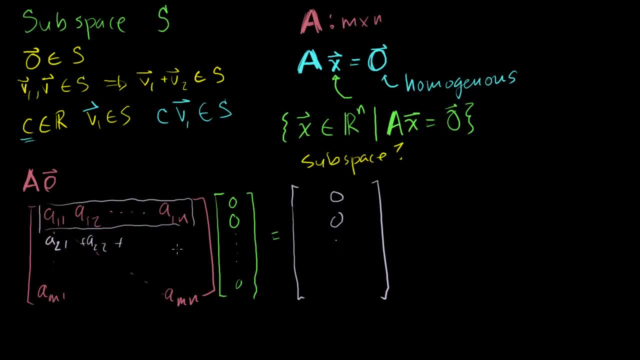 well, I haven't defined dot products with row vectors and column vectors, but I think you get the idea: The sum of each of these elements multiplied with the corresponding component in this vector, And of course you're just always multiplying by 0 and 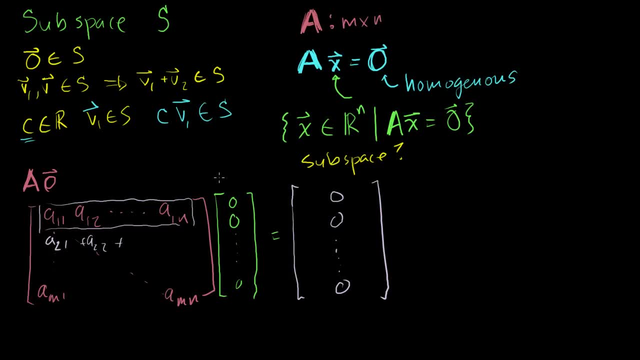 then adding up, So you're going to get nothing but a bunch of 0's. So the 0 vector does satisfy the equation. a times the 0 vector is equal to the 0 vector, And this is a very unconventional notation. 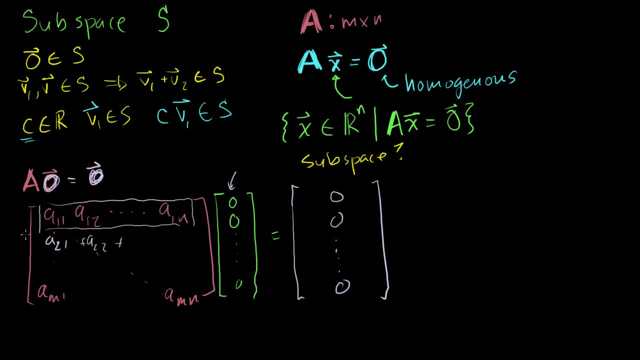 I'm just writing it like that because I don't feel like bolding out my 0's all the time to make you realize that that's a vector. So we meet our first requirement: The 0 vector is a member of this set. 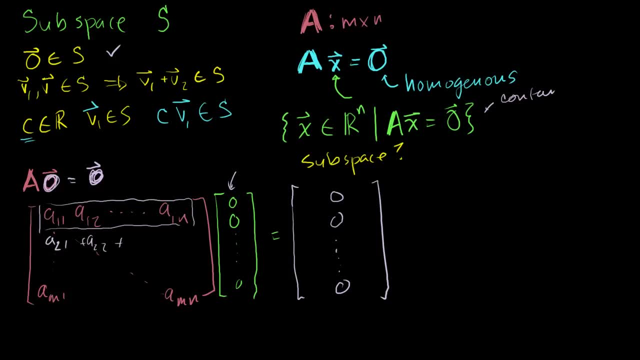 So it does contain. so let me define my set here. Let me define it n, And I'll tell you in a second why I'm calling it n. So we now know that the 0 vector is a member of my set n. 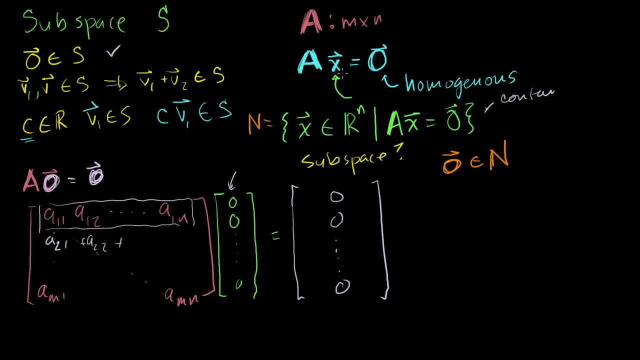 Now let's say I have two vectors, v1 and v2, that are members. let me write this: So let's say I have two vectors, v1 and v2, this was a v2 over here- v1 and v2, that are both members of our set. 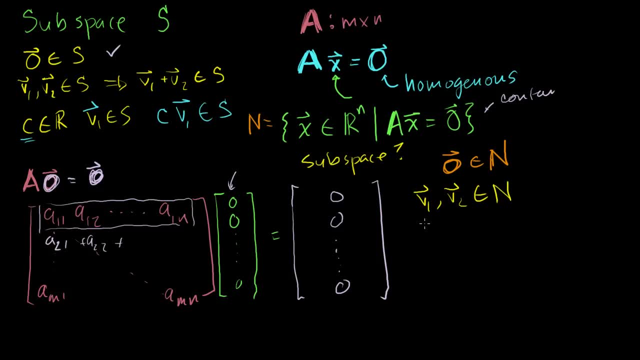 What does that mean? That means that they both satisfy this equation. So that means that a My matrix a times vector 1 is equal to 0. This is by definition. I'm saying that they're a member of this set, which means: 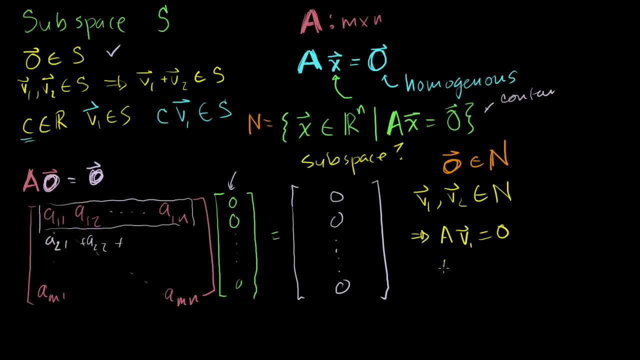 they must satisfy this, And that also means that a times vector 2 is equal to our 0 vector. So in order for this to be closed, under addition, a times vector 1 plus vector 2, the sum of these two vectors should: 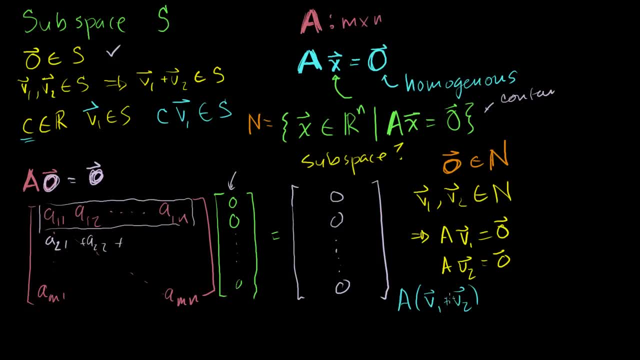 also be a member of n, But let's figure out what this is. Let's figure out what this is: The sum of these two vectors is this vector right here? This is equal to- and I haven't proven this to you yet. 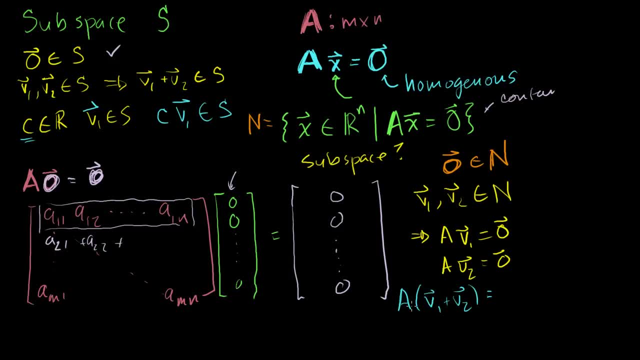 I haven't made a video where I prove this, but it's very easy to prove, just using the definition of matrix vector multiplication, that matrix vector multiplication does display the distributive property, And maybe I'll make a video on that. but literally you just 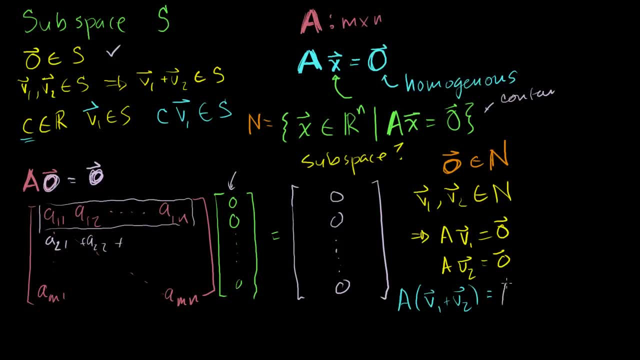 have to go through the mechanics of each of the terms. This is equal to a v1 plus a v2.. And we know that this is equal to the 0 vector, and this is equal to the 0 vector. And if you add the 0 vector to itself, this whole thing is. 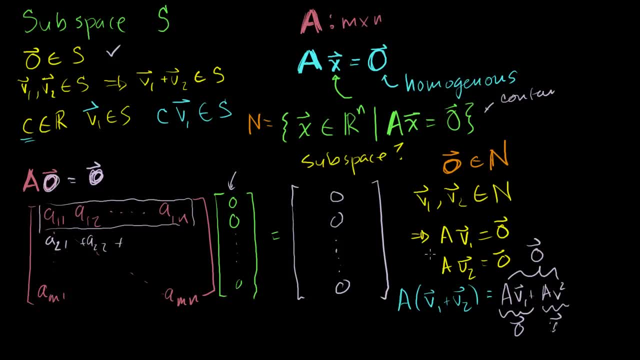 going to be equal to the 0 vector. So if v1 is a member of n and v2 is a member of n, which means they both satisfy this equation, then v1 plus v2 is definitely still a member of n, because when I multiply a, 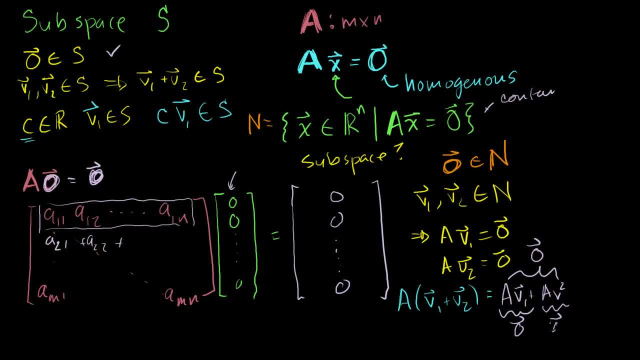 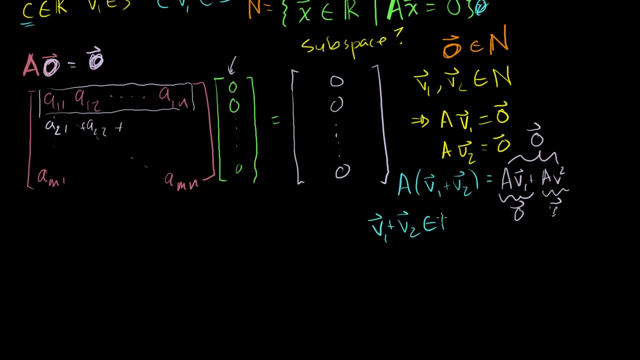 times that I get the 0 vector again. So we get. let me write that result as well. So we are also. let me write that. so we are. also. let me write this. Let me write this right here. So we now know that v1 plus v2 is also a member of n. 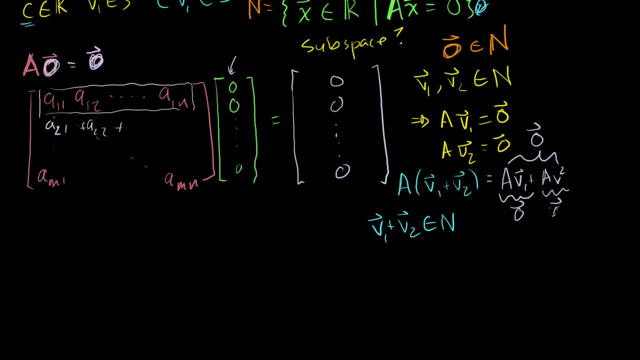 And the last thing we have to show is that it's closed under multiplication. So let's say that v1 is a member of our space that I defined here, where they satisfy this equation. What about c times v1?? What about c times v1?? 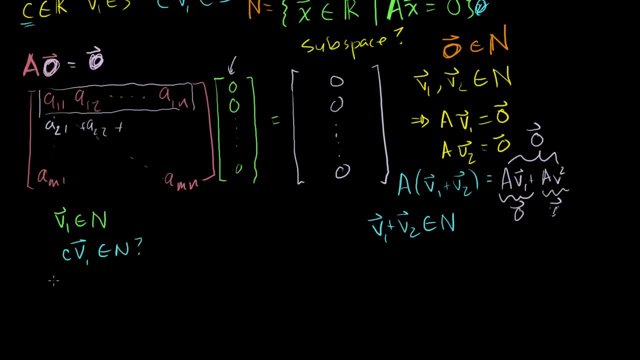 Is that a member of n? Well, let's think about it. What's A, our matrix, A times the vector, right? I'm just multiplying this times the scalar. I'm just going to get another vector. I don't want to write a capital V there. 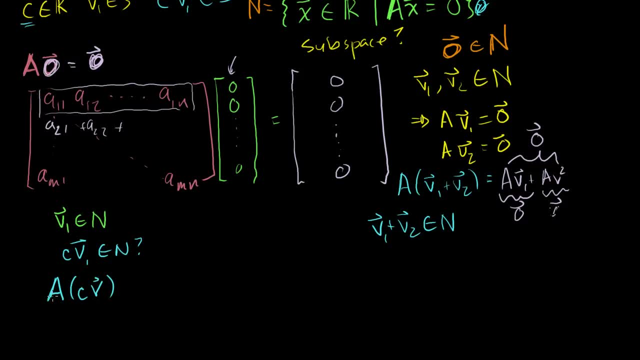 Lowercase v, so it's a vector. So what's this equal to? Well, once again, I haven't proven it to you yet, but it's actually a very straightforward thing to do to show that when you're dealing with scalars. if you have a scalar here, it 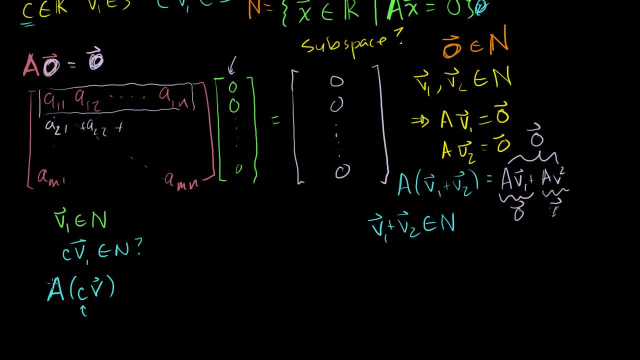 doesn't matter if you multiply the scalar times the vector before multiplying it times the matrix, Or multiply it times the matrix, Or multiplying the matrix times the vector and then doing the scalar. So it's fairly straightforward to prove that this is equal to. 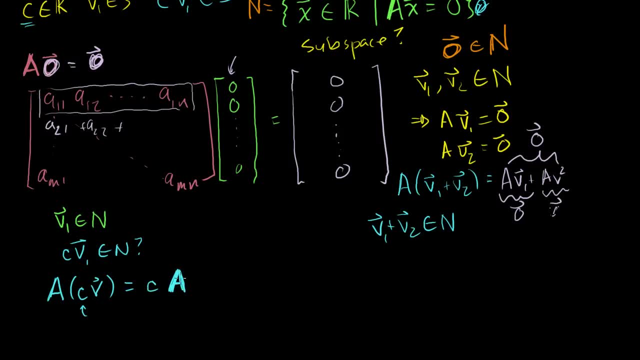 c times our matrix A- I'll make that nice and bold- times our vector v, That these two things are equivalent. Maybe I should just churn out the video that does this, but I'll leave it to you. You literally just go through the mechanics by component and 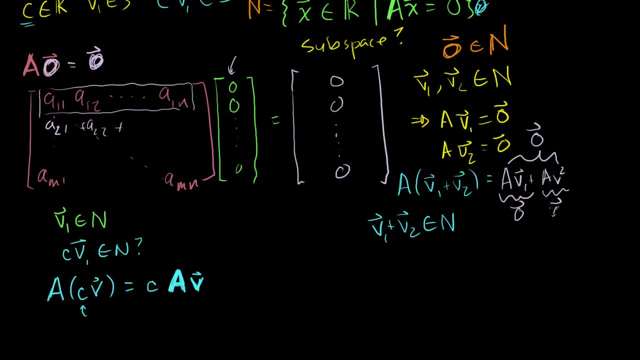 you show this, But clearly, if this is true, we already know that v1, sorry, this was v1.. We already know that v1 is a member of our set, which means that A times v1 is equal to the 0 vector. 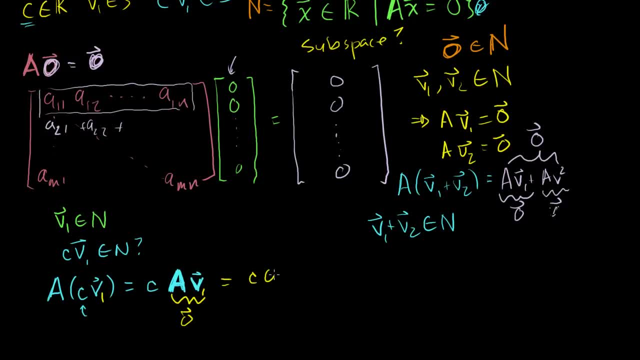 And so that means. well, this will reduce to c times the 0 vector, which is still the 0 vector. So cv1 is definitely a member of n. So it's closed under multiplication, And I kind of assumed this right here, but maybe I'll. 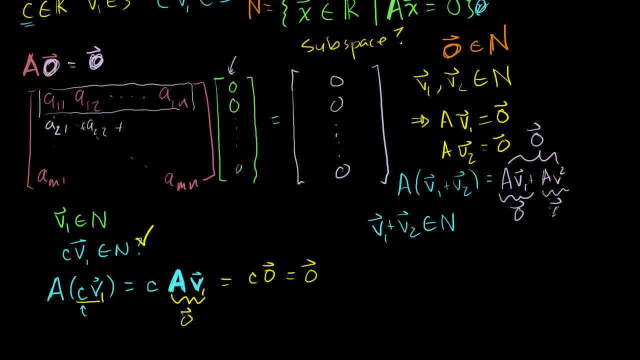 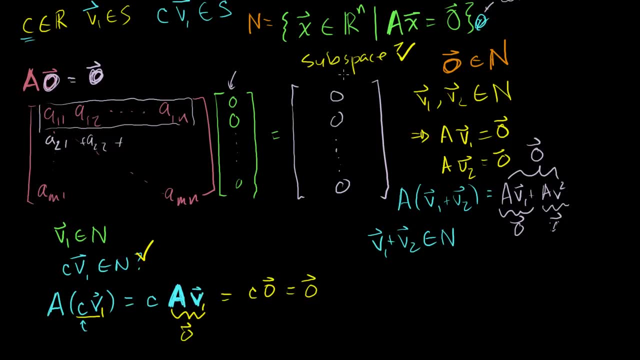 prove that in a different video. But I want to do all of this to show that this set n is a valid subspace. This is a valid subspace. It contains the 0 vector. It's closed under addition. It's closed under multiplication. 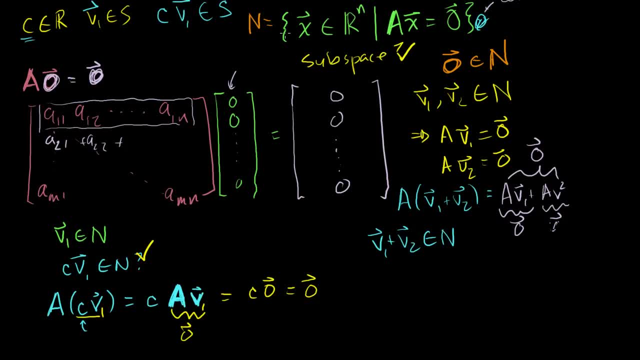 And we actually have a special name for this. We call this right here. we call n. the null space of A, Or we could write n, is equal to. maybe I shouldn't have written an n. maybe I'll write an orange n there. 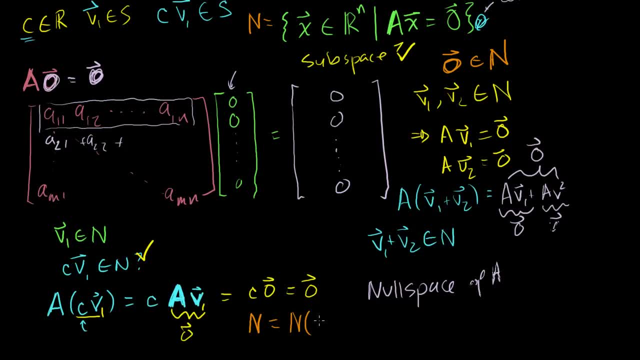 n is equal to the notation, is just the null space of A. Or we could write: the null space is equal to the orange notation of n. And so literally, if I just give you some arbitrary matrix A and I say, hey, find me n of A, what is that? 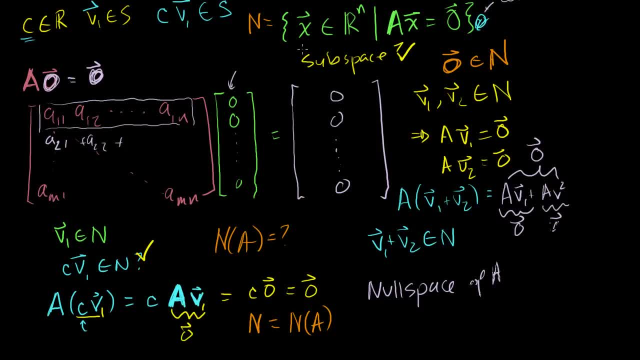 You, literally. your goal is to find the set of all x's that satisfy the equation A times x is equal to 0. And I'm going to do that in the next video.